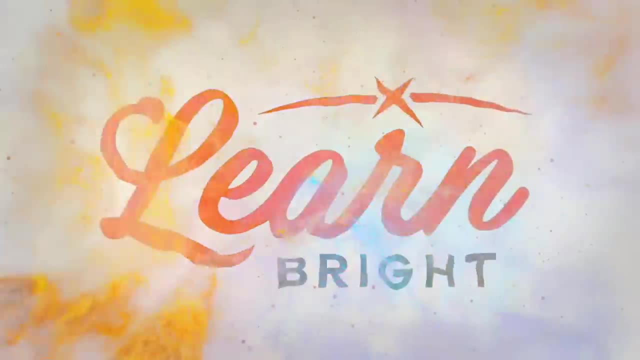 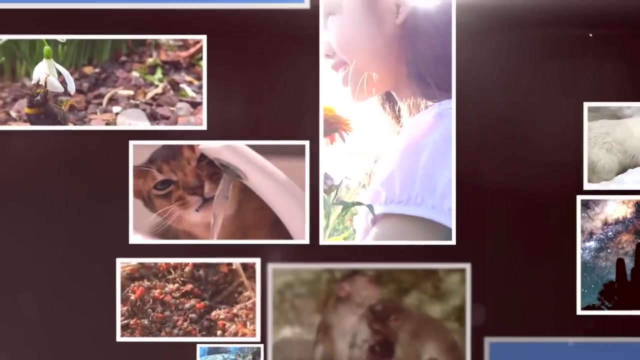 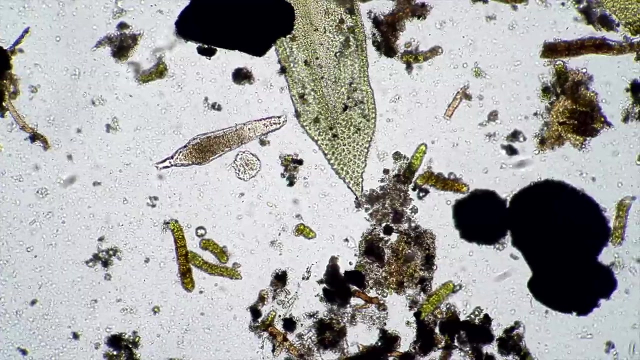 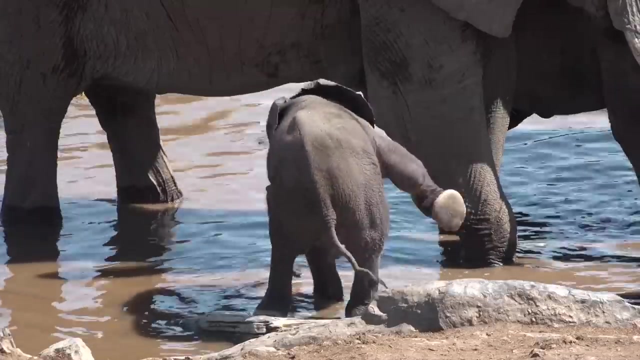 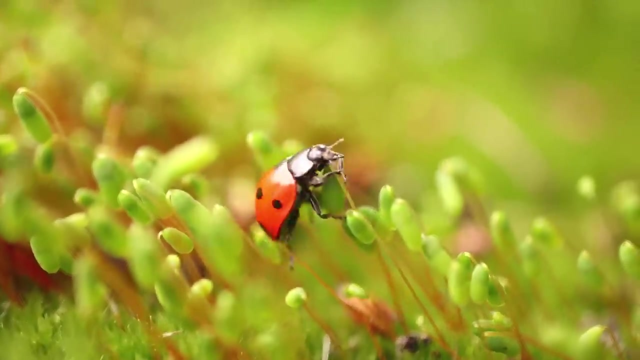 Habitats for Kids. Did you know that you have something in common with all the other life forms on Earth? Seriously, even down to the tiny microorganisms our eyes cannot see, Ready to find out what it is. We all live in habitats. Today, we are going to take a journey through some of these habitats and learn more about them. 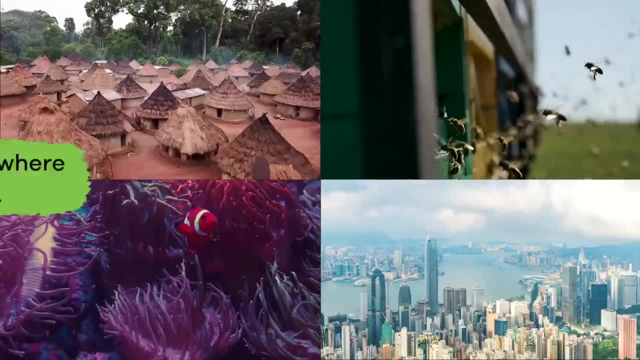 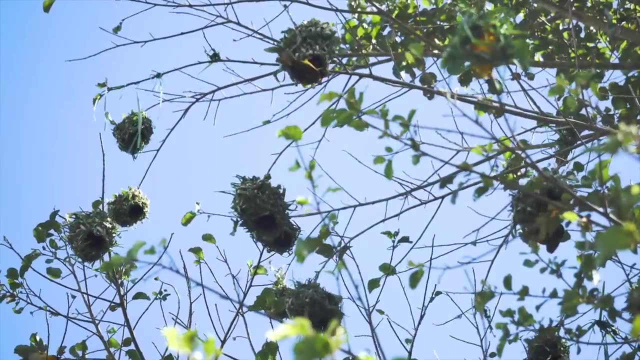 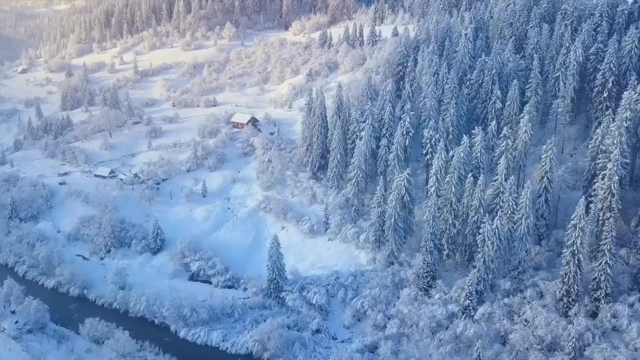 But first, what is a habitat? Habitats are places and environments where a living organism makes its home, And they provide everything a living thing needs for survival. No matter where you live, it is your habitat. A habitat can be large or small. 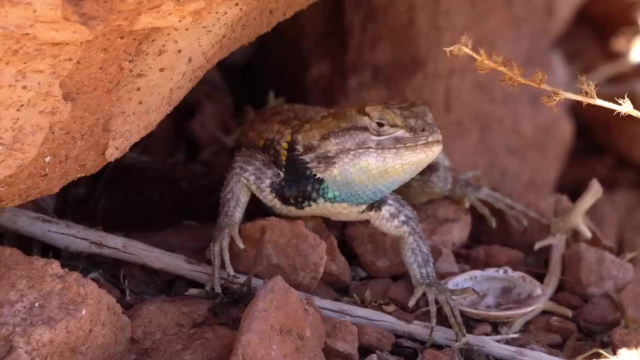 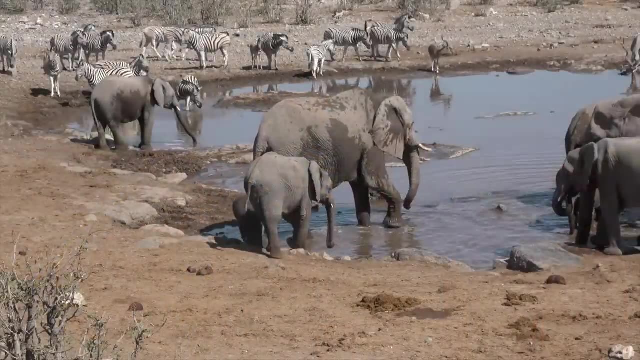 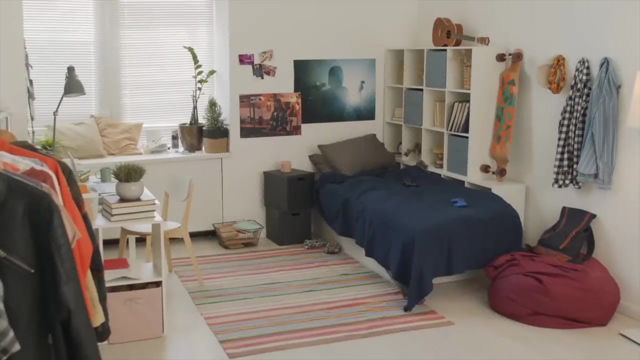 An entire continent or the space underneath a single rock. These environments usually have lots of different kinds of organisms living together and includes non-living things that also exist in the habitat. For example, your bed is not a living thing, but it is definitely a part of your habitat. 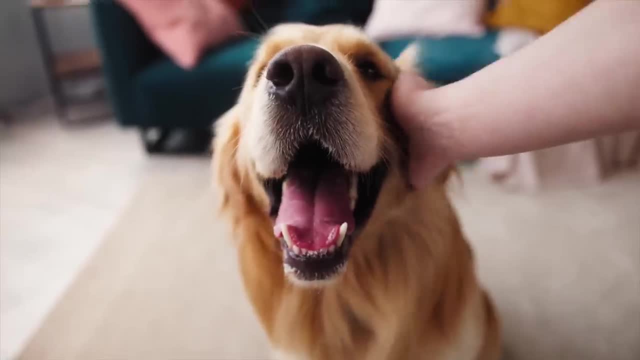 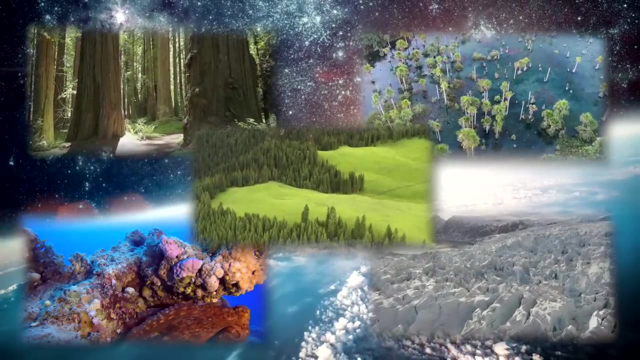 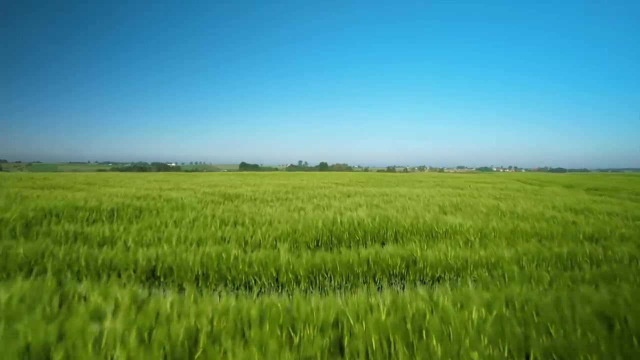 And some living things can live in more than one habitat. There are many different kinds of habitats. There are many different kinds of habitats that can be found on Earth. Let's talk about a few. First up are grasslands. A grassland is full of tall growing grass and does not have a lot of trees. 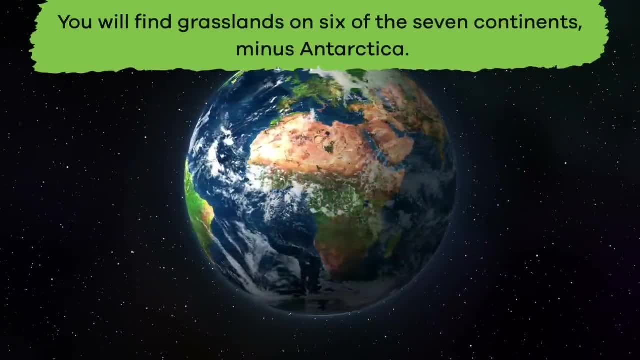 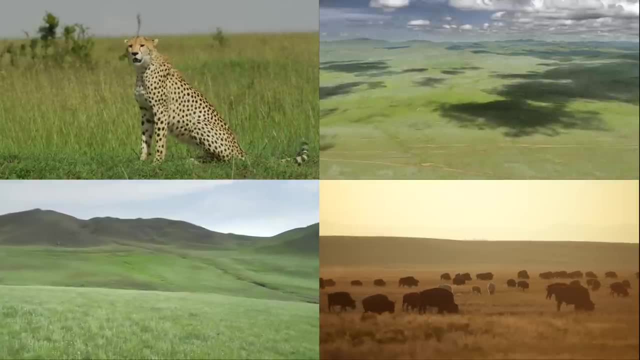 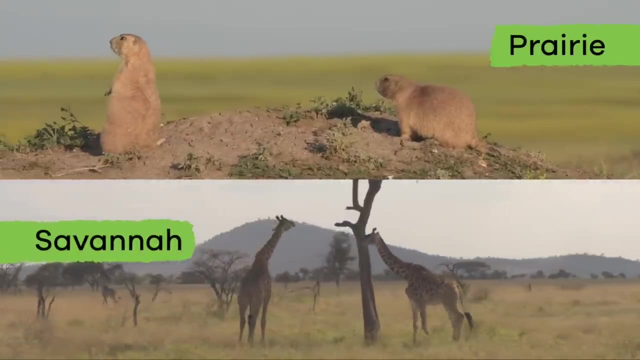 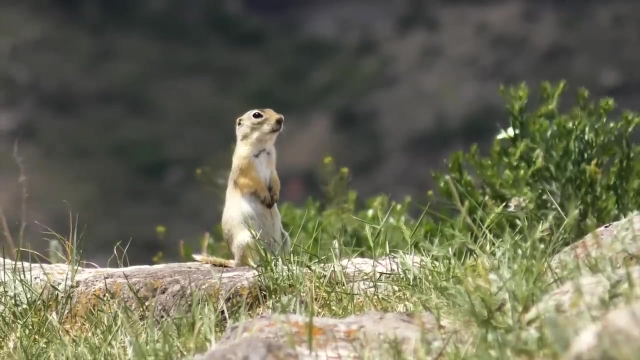 You will find grasslands on six of the seven continents minus Antarctica. Here is an interesting fact: There are different types of grasslands. Prairies and savannas are two of these different kinds. Animals like aardvarks, antelope, brown bears, squirrels, lions and hippos can all live in this kind of habitat. 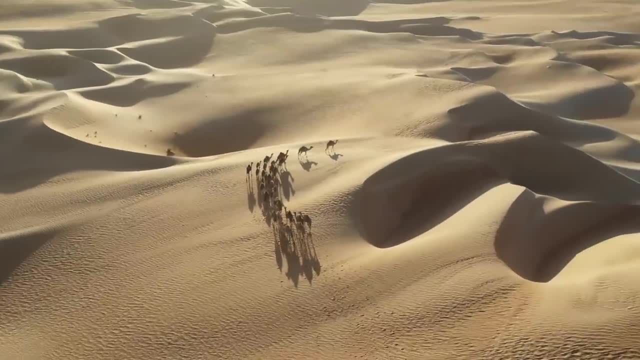 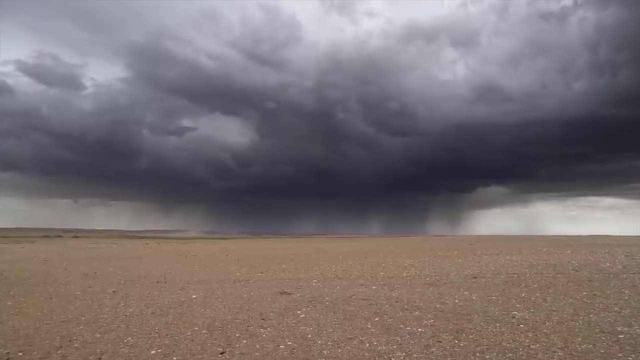 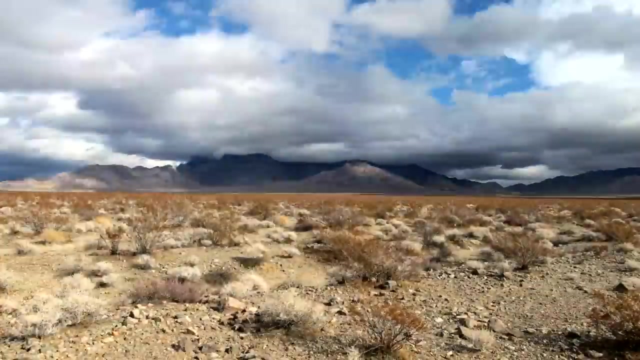 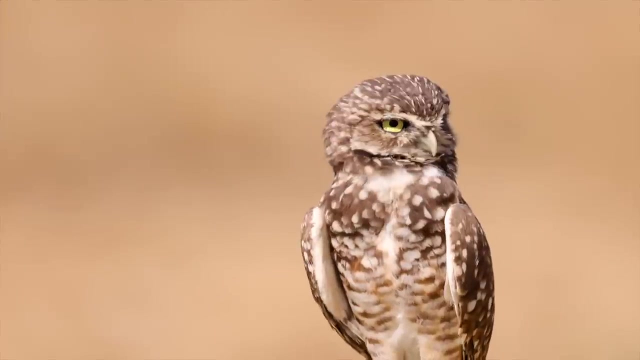 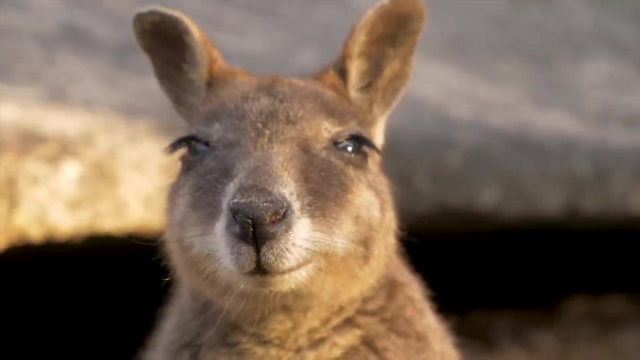 Now let's travel to the desert. A desert is extremely dry, can be hot or cold, and gets less than six inches of rain per year. Deserts are found everywhere on the planet. There is little plant life, but animals like snakes, lizards, birds, camels, kangaroos and more. all can survive in the desert. 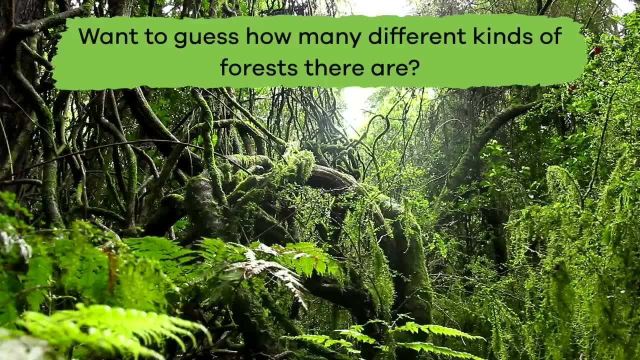 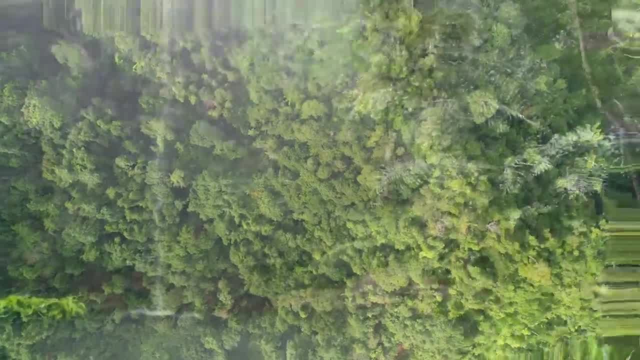 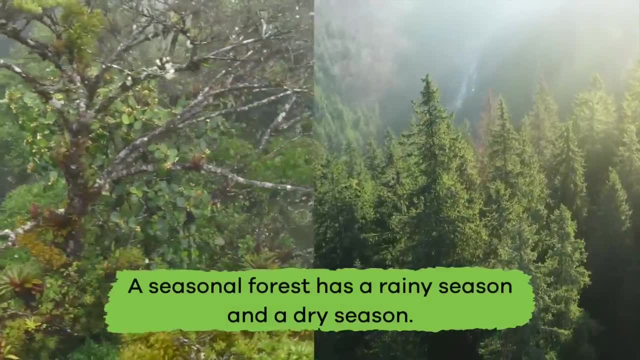 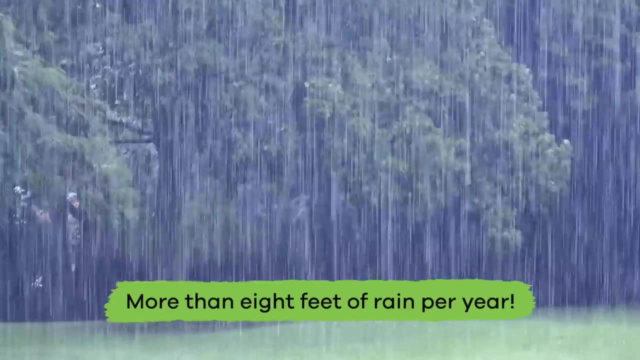 Want to guess how many different kinds of forests there are So many. Let's begin with tropical forests. A rainforest gets rain all year long, While a seasonal forest has a rainy season and a dry season, But both of these types of forests receive more than eight feet of rain per year. 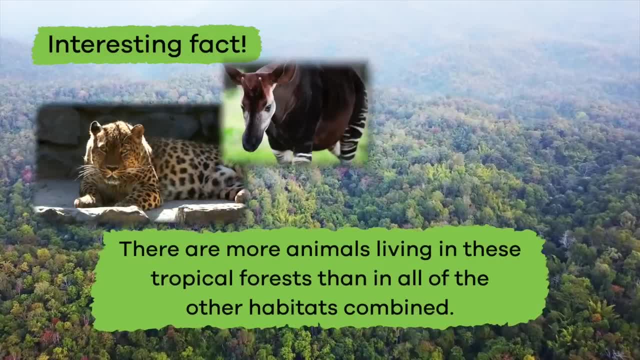 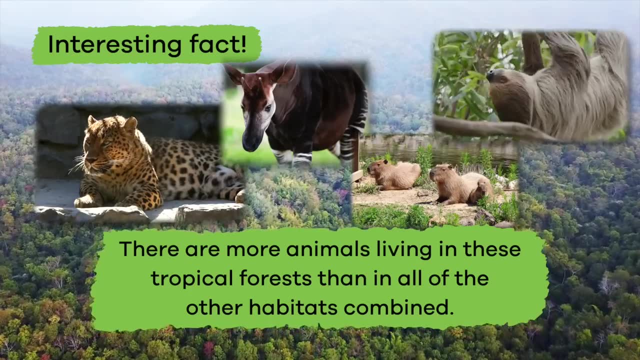 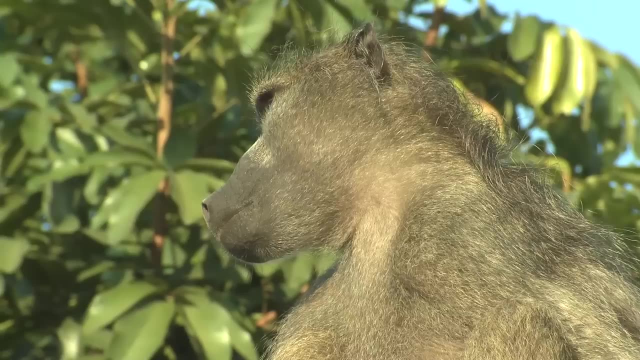 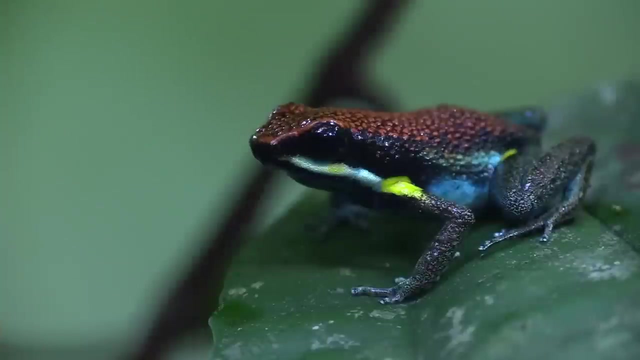 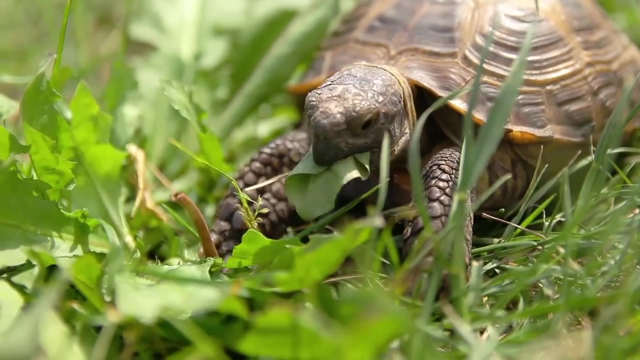 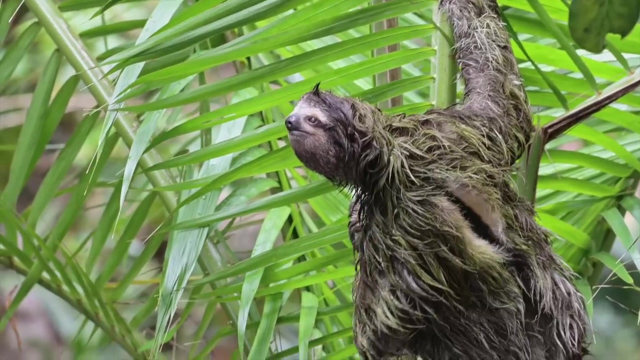 Here is another interesting fact: There are more animals living in these tropical forests than in all of the other habitats combined Wild right. If you are in a tropical forest, you are more than likely to find animals like baboons, Bats, butterflies, geckos, frogs, monkeys, tigers, toucans, tortoises, ladybugs, elephants and crocodiles, and so many more. 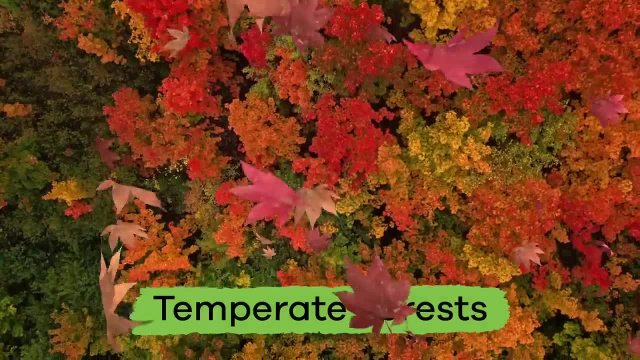 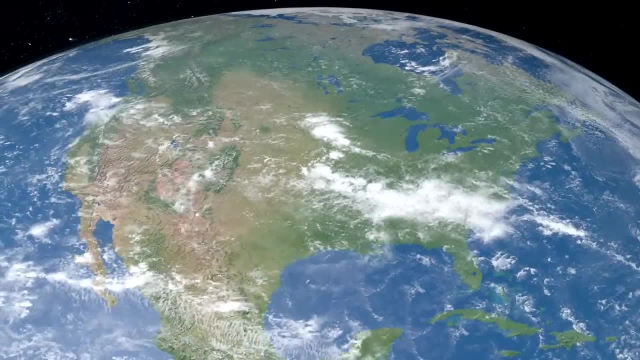 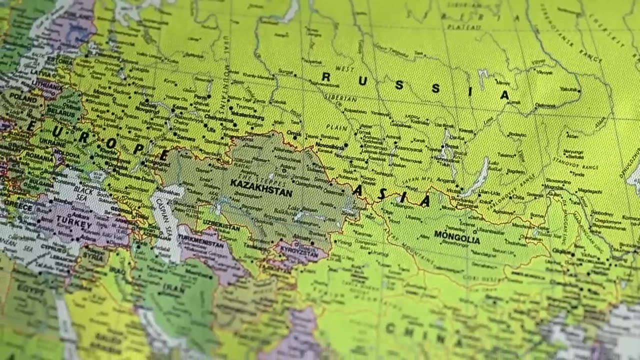 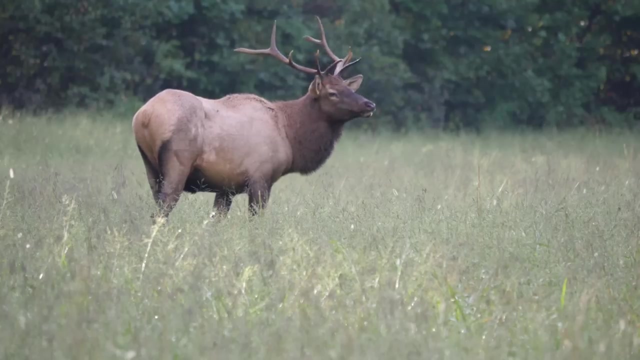 Temperate forests have trees that lose their leaves in the winter or remain green all year long, Like pine trees. There are lots of temperate forests found in the United States and on other continents like Europe and Asia. This is the habitat where you can find deer elk, turkeys and wolves. 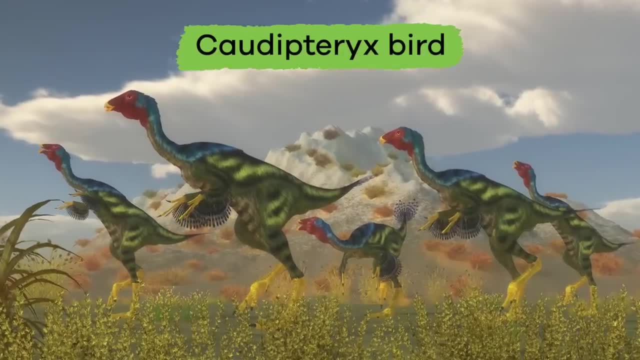 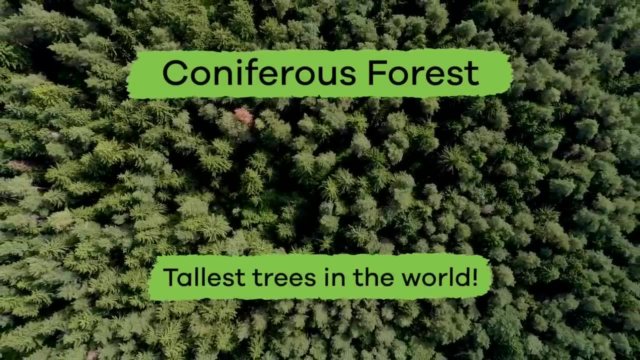 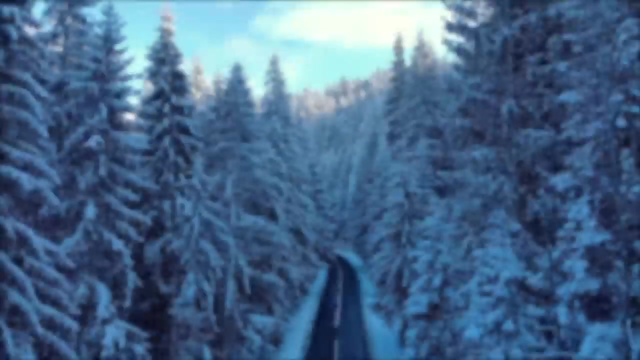 And guess what? Way back in the day, dinosaurs used to live in temperate forests too. The coniferous forest is where the tallest trees in the world grow. These trees are very strong and can survive extremely cold temperatures. Many animals call this habitat home. 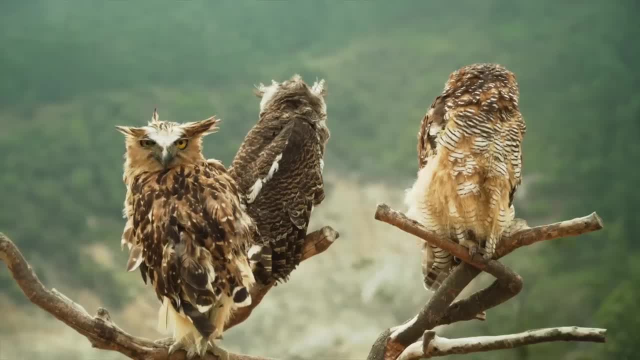 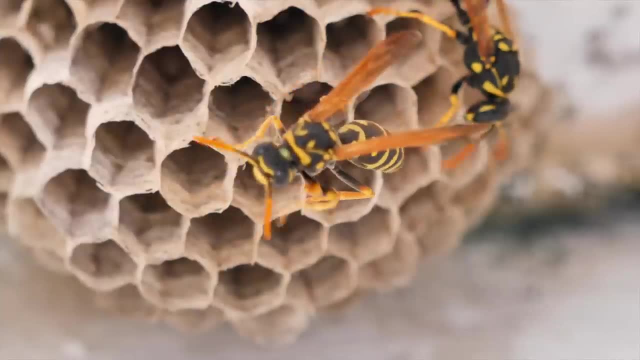 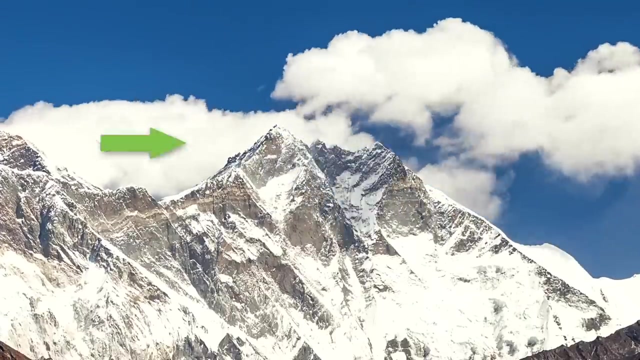 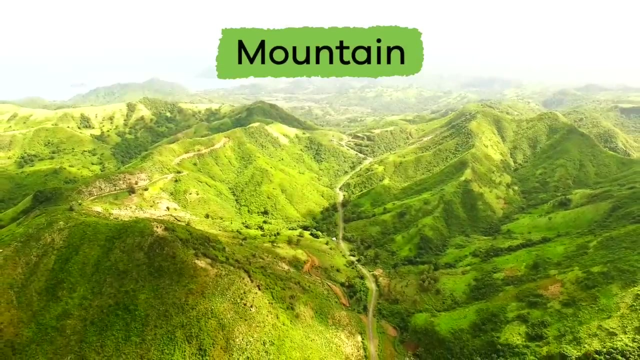 Animals like eagles, owls, raccoons, giant pandas, weasels, wasps and worms. Our Earth is pretty amazing. Hey, what is that over there? That's right, it's a mountain, And mountains are another kind of habitat. 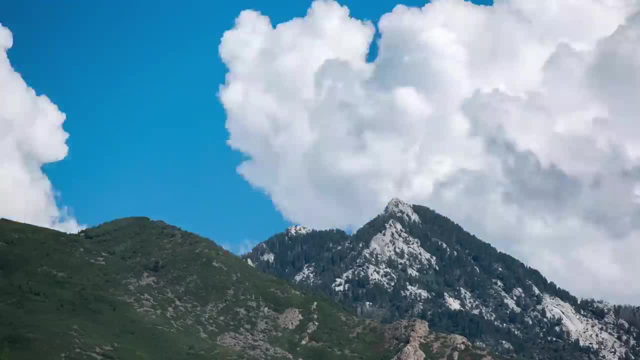 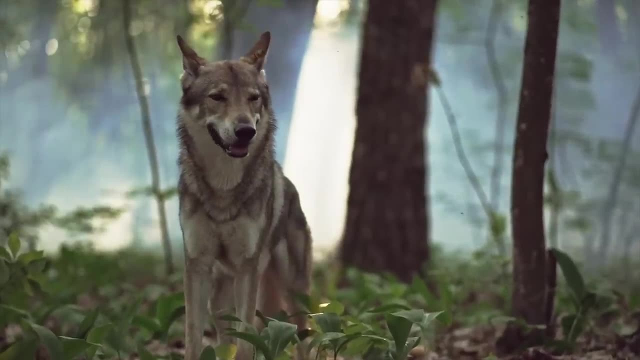 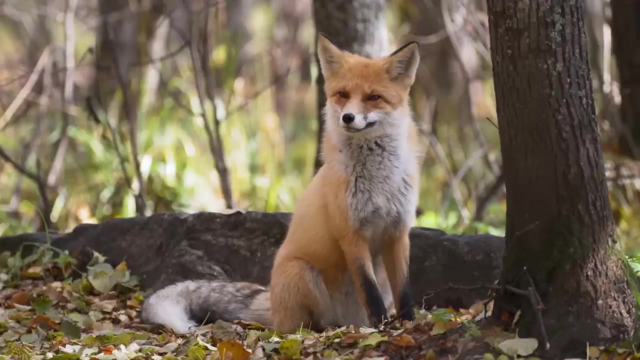 The temperature up high is much cooler and the oxygen is much thinner than in places closer to the ground, But there are still animals that live there, Creatures like badgers, beavers, buzzards, foxes, red pandas, wombats, wrens. 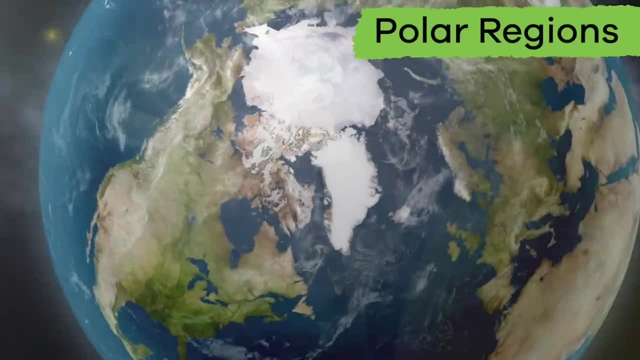 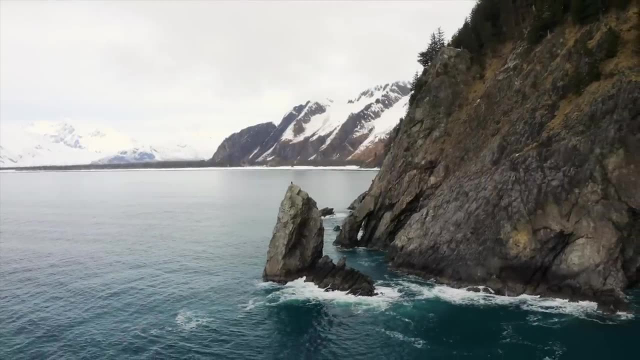 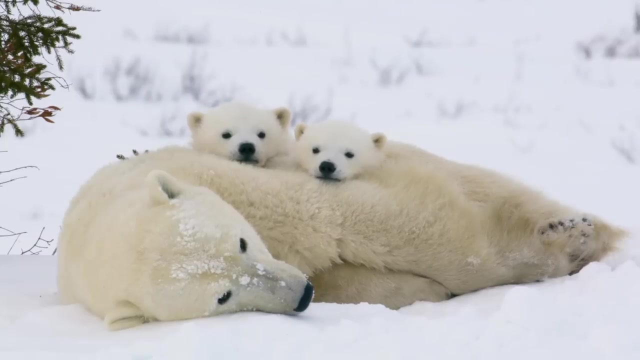 and gorillas. The polar regions are the coldest places in the world And the land is partly frozen. As you probably already guessed, these habitats are found at the north and south poles of the Earth. Animals like polar bears, penguins, 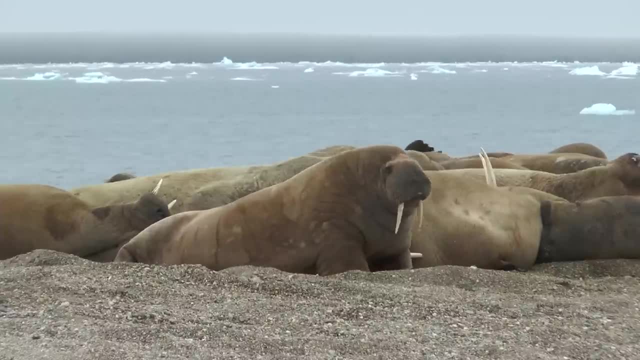 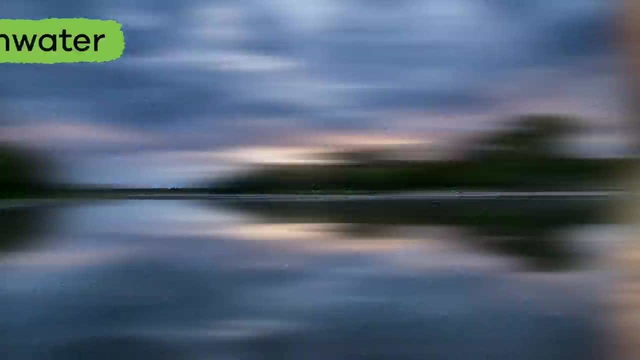 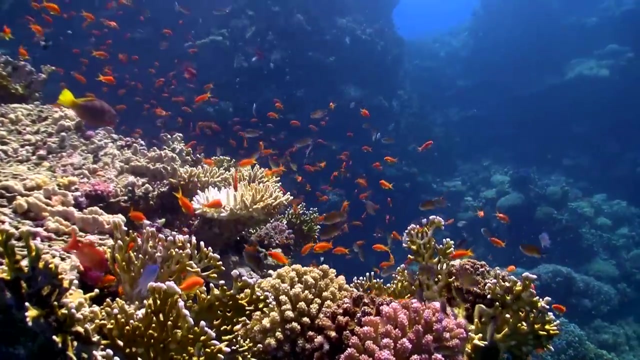 whales and walruses live there. Habitats are not just found on land. Freshwater sources like lakes, streams and rivers, and saltwater-filled oceans with their coastlines and coral reefs, are also habitats. Freshwater habitats are home to many reptiles. 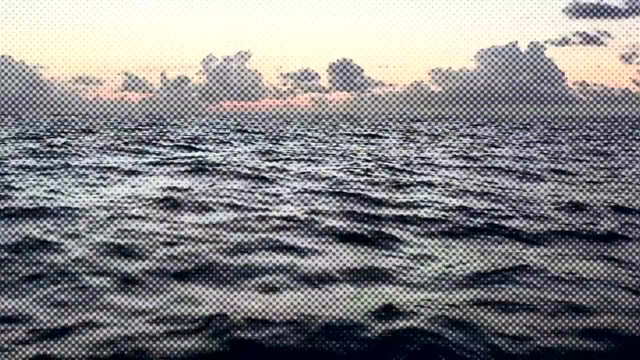 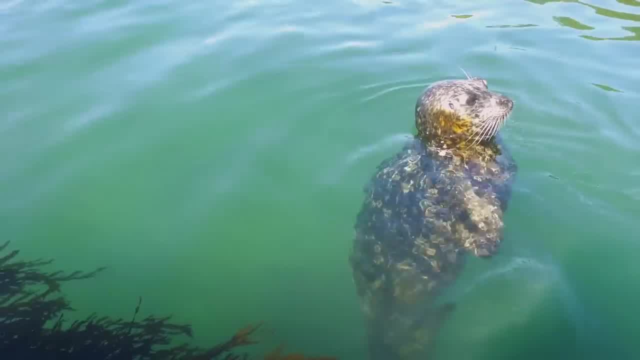 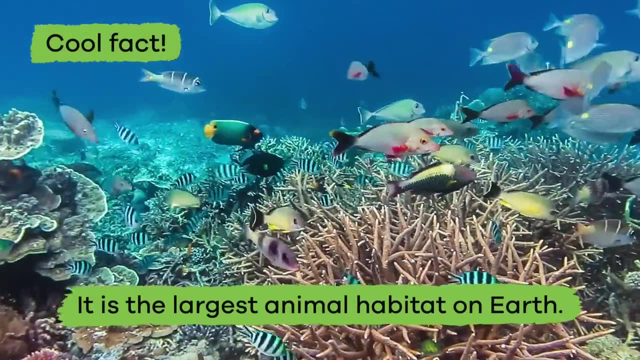 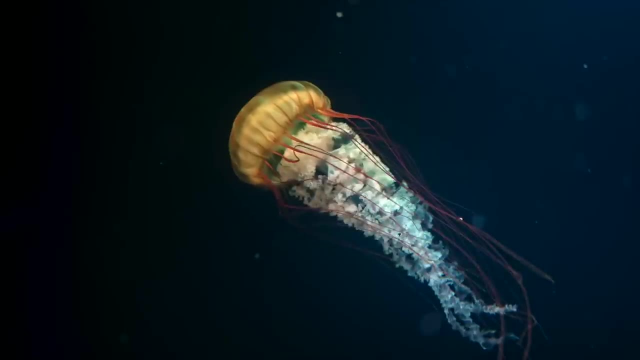 fish and birds, And oceans are home to creatures like lobsters, orcas, seals and sharks. Here is a cool fact about the ocean: It is the largest animal habitat on Earth. It is so large that there are some parts that have never been explored by humans. 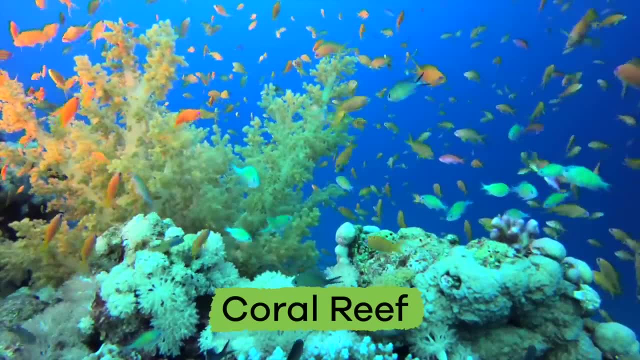 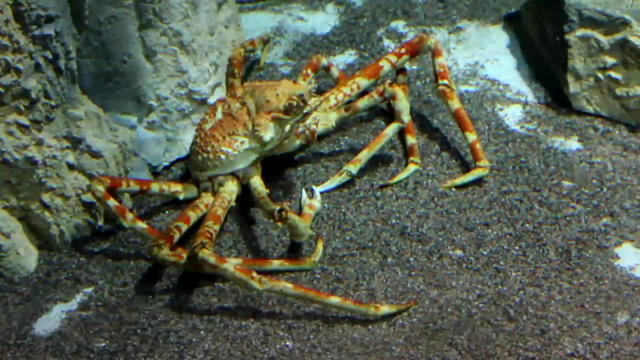 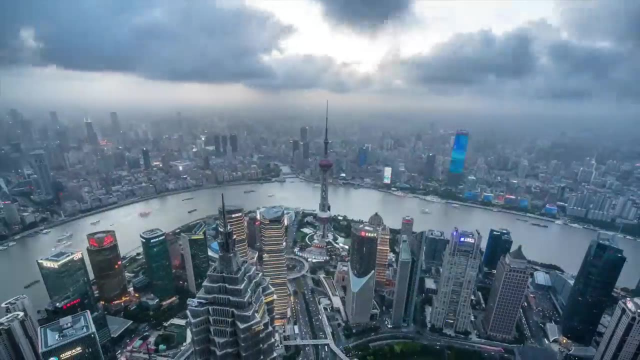 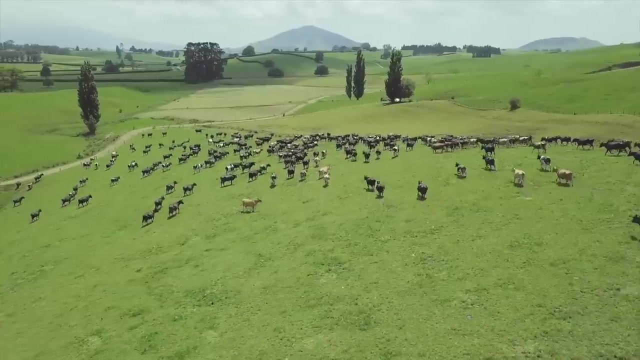 Coral reefs are like a habitat within a habitat and need sunlight to survive. Reef animals include crabs, eels, clams and angelfish. Last but not least, we have cities and farms, After talking about all of these other kinds of habitats. it might seem strange to include these last two, But they are both just as important. In fact, they just might be. the habitats you live in. Cities are home to humans, pets, bugs and other small mammals, and birds. Farms too.